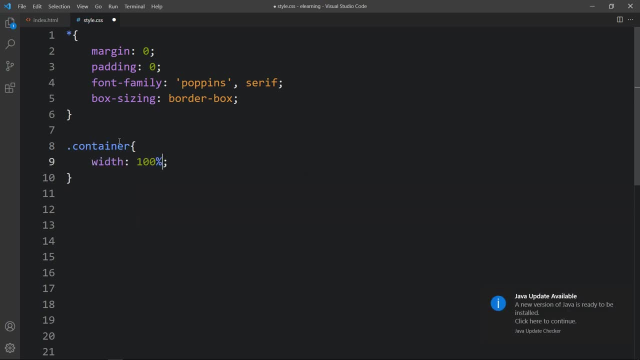 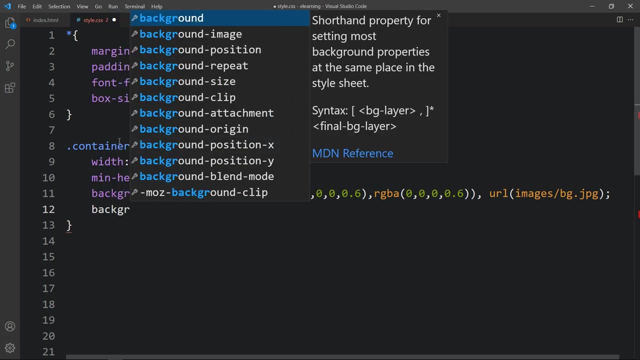 in the css file and for this one we will add some css properties, like we will add width, min height, then we will add background and in this background we will add linear gradient, color and one image. this is the image file path: images- bgjpg. then we will add background. 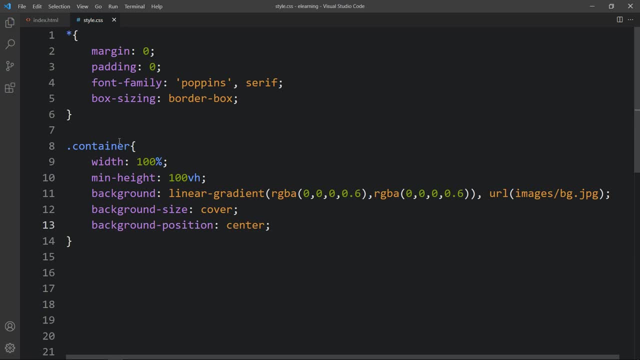 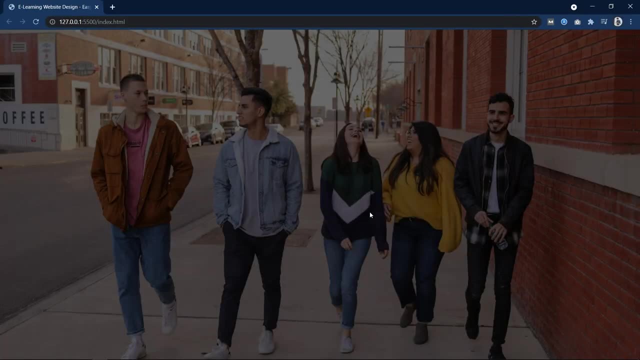 size and background position. now we will open our web page with web browser. here i will select open with live server. so right now you can see one image on complete web page and there is a dark layer on this image. let's come back and in this div we will create one. 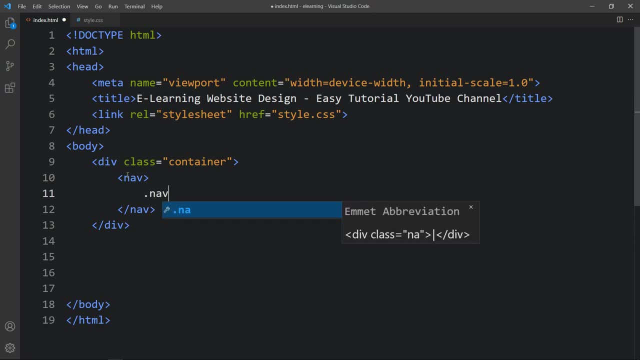 nav tag and here let's create one div with the class name nav logo and in this one we we will add one logo. so i am using the img tag, image file path, and after that we will create another div. so let's add the class name nav links in this nav links. we will add one link in a tag. 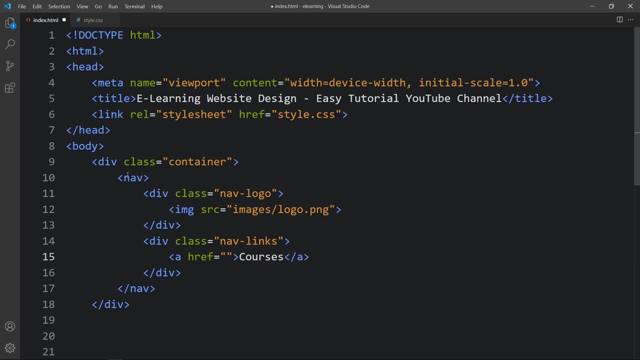 so link text will be courses. after that we will create another div and in this div let's create a link and the link text is login. let me duplicate it. and the link text is sign up. so we have total three links in the navigation bar. let's open the website again and you can see this logo and three. 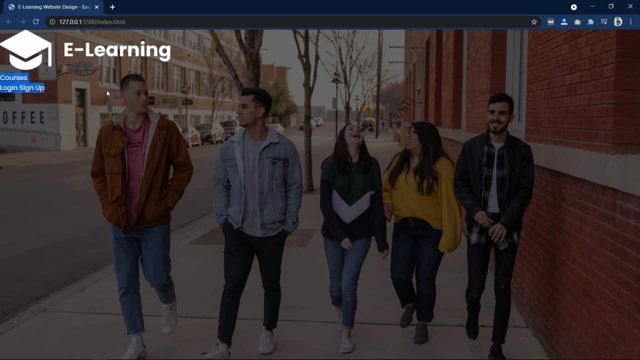 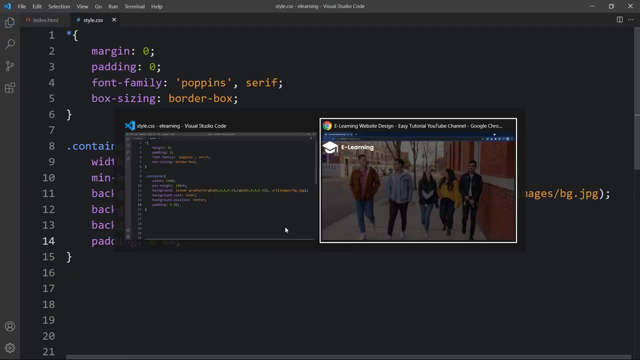 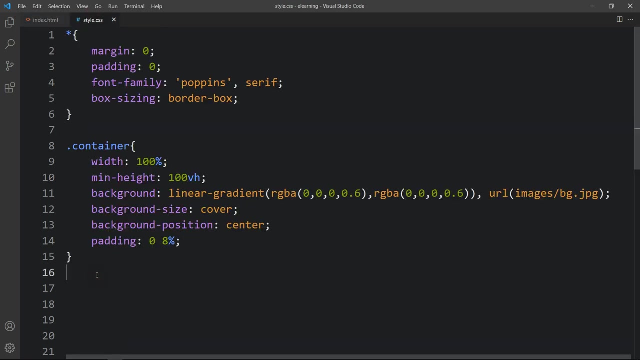 links: courses: login- sign up. let's come back and come to the css file. here in this container we will add padding. let me add zero and eight percent. now you can see some space from the left side. now let's come back and copy this nav, write it here and here we will. 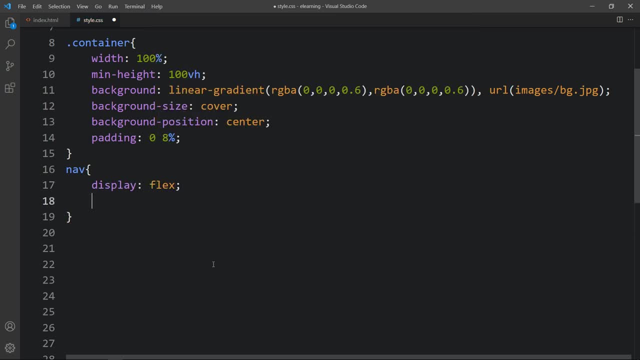 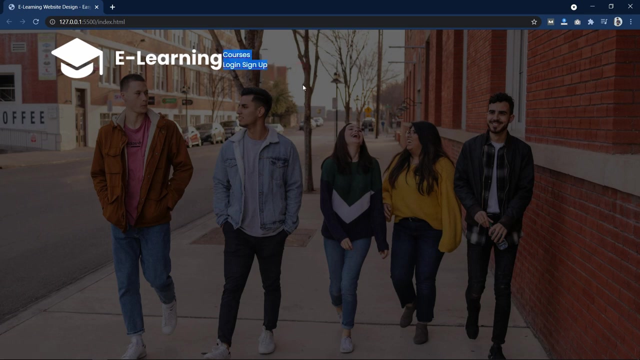 add the css properties for this nav tag. let me add display, flex align item center and flex wrap wrap. then we will add some padding. and let's come back to the website and you can see this link is over here. let's come back and copy this class name nav logo, write it here and after that we will add. 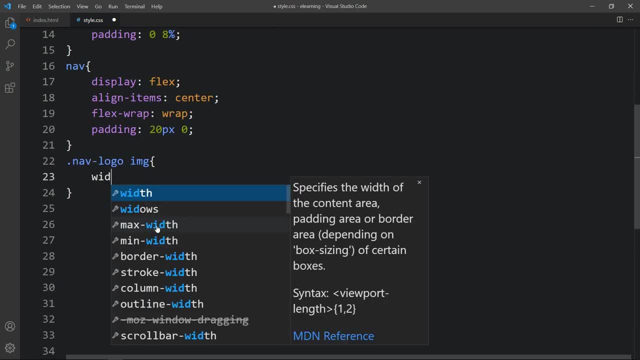 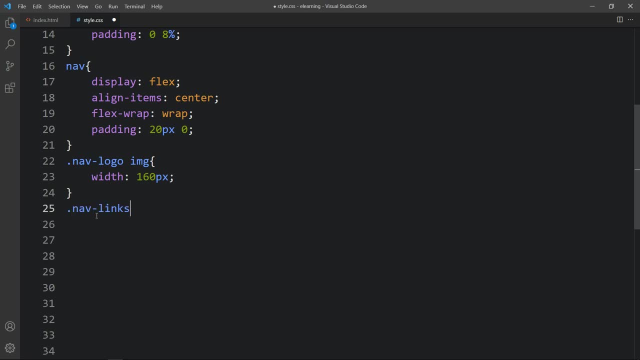 img, because we have one image in this div, so here we will add width: 160 pixel. let's come back and copy this class name, nav logo, and here we will add one image in this div, so here we will add another class name, which is nav links. for this nav links we will add display flex, then we will 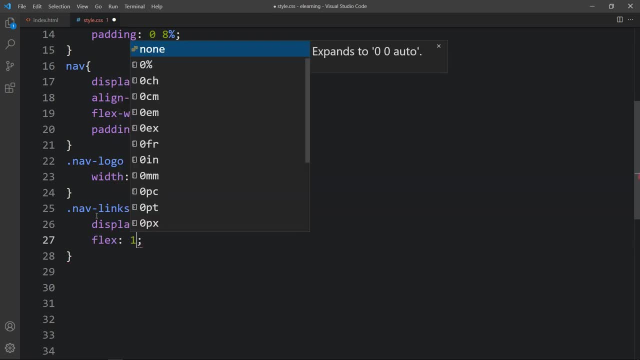 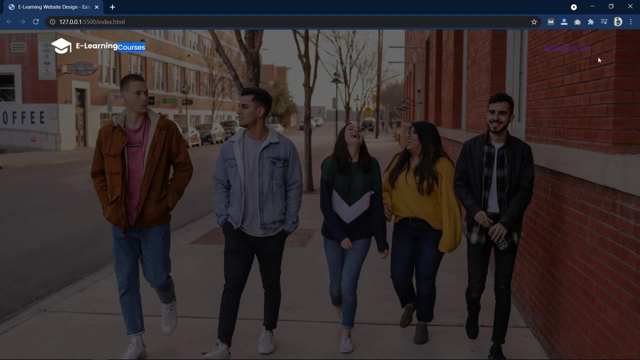 add flex one so it will use the entire space available in the row. then we will add align item center and justify content. it will be space between- now you can see this course link in the left side and two other links in the right side because of justify content. space between, let's. 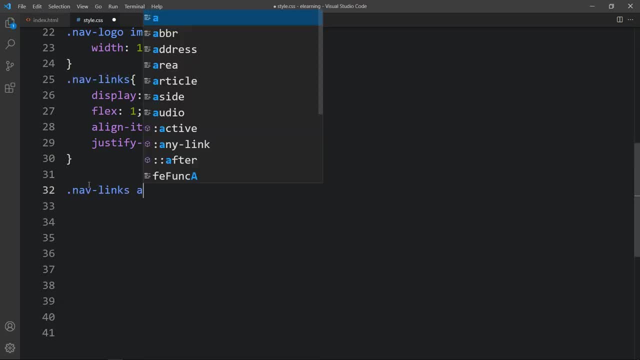 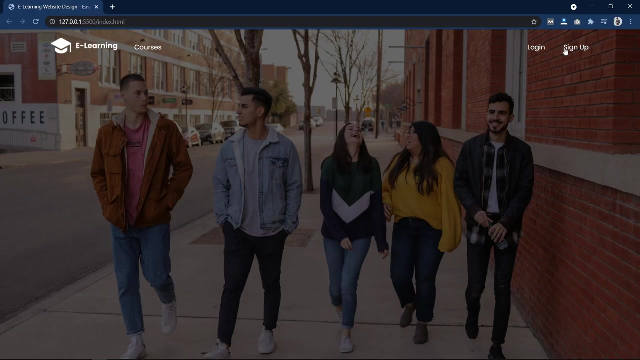 come back and copy this nav links again, and here we will add a for this a tag. we will add text, decoration: none, and we will add color, so it is white. then we will add some margin from the left side so there will be some space between the links. now it looks good. 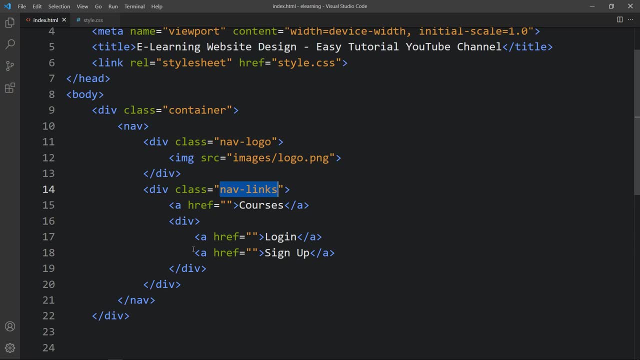 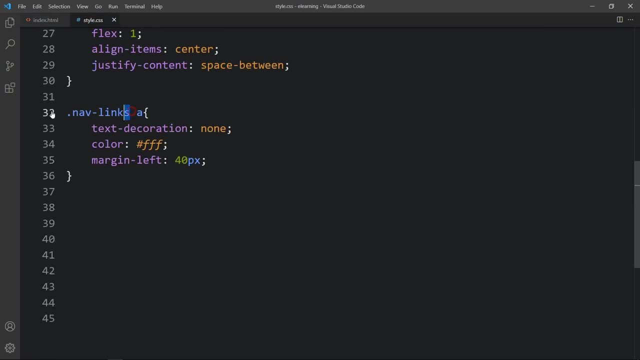 next we will design the last link. so let's come back and here we will add class name btn. next we will add the css properties for this. so just come back and write this class name, nav links. then write btn for this button. we will add background and color. after that we will add some padding and border radius. 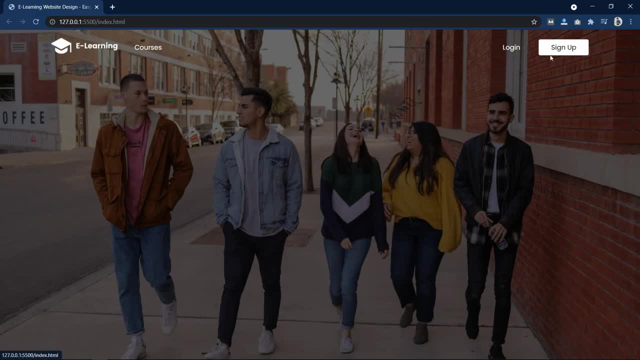 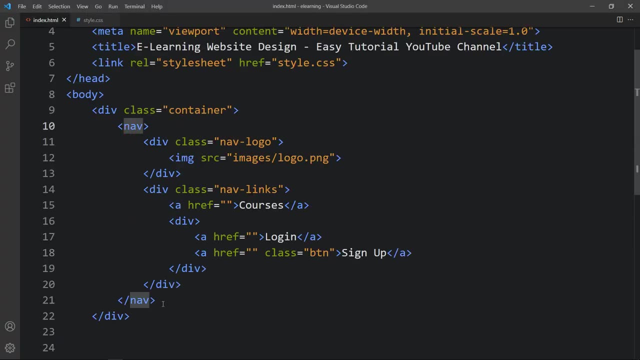 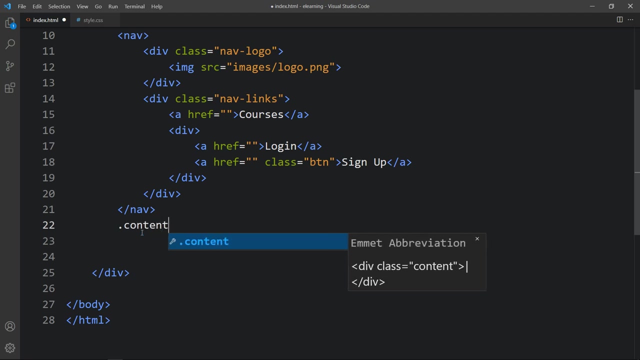 for pixel. now this button looks good, so let's come back to the html file again, and after this nav tag we will create another div. so let me create a div with the class name content, and in this one we will add one title. so let me add the title in h1 tag and the title is: 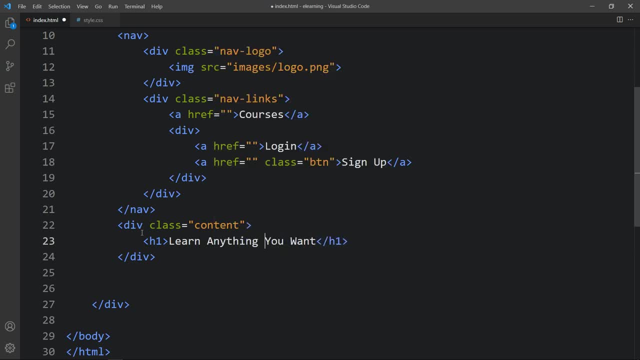 learn anything you want here. we will add br to add a line break. after that we will add one search box. so let me add a div with the class name search box. in this search box we will add one input box. type will be text, then placeholder search- any course, then we. 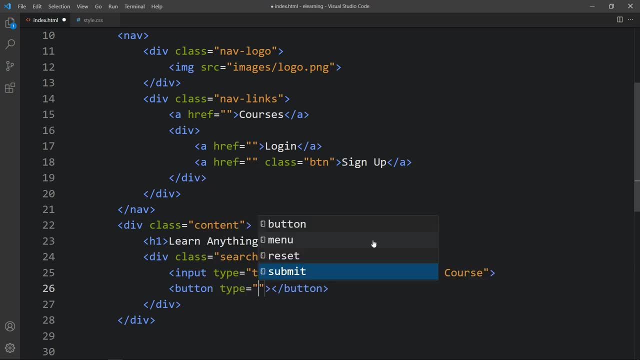 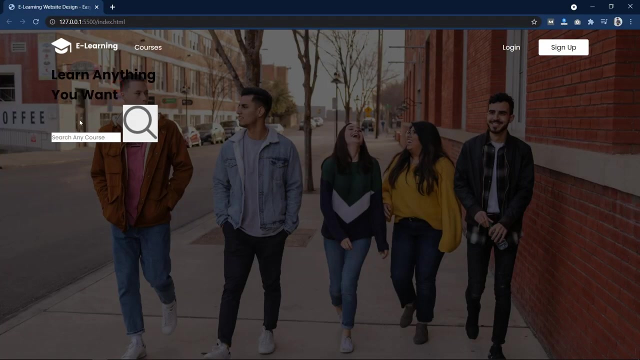 will add one button, type will be submit, and in this button we will not add any text. we will add one image and the image file path is images slash, searchbat png, which is a search icon. after applying this, you can see this text: one input box and this: 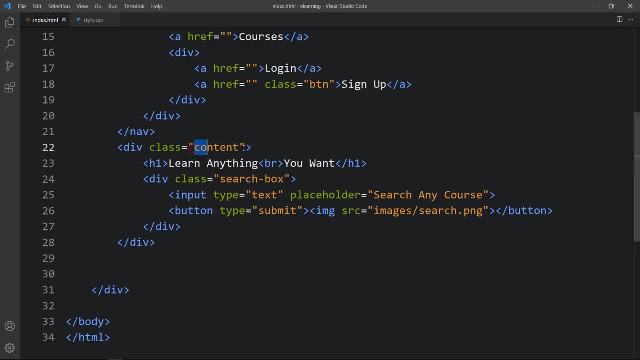 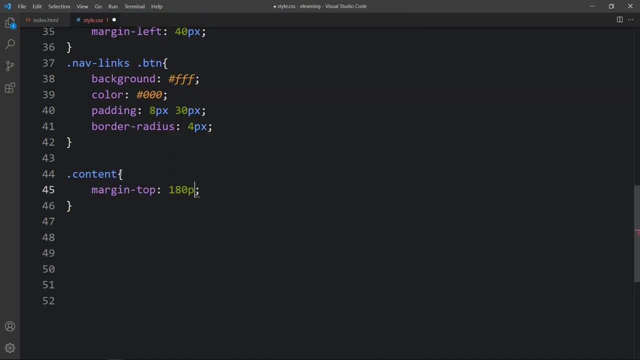 search icon. next we have to design it. so let's come back and copy this class name content. write it here in this css file. for this content we will add some space from the top, so we will add margin top. then we will add color. it will be white. then write this class name again. 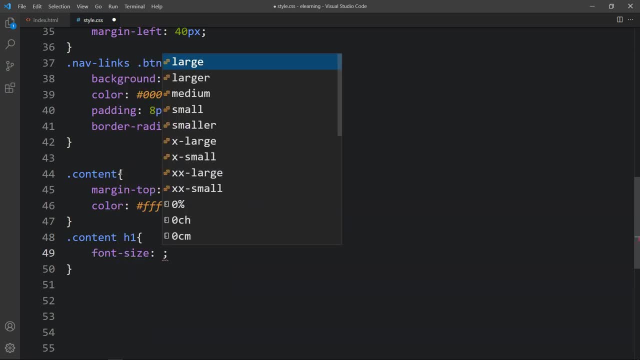 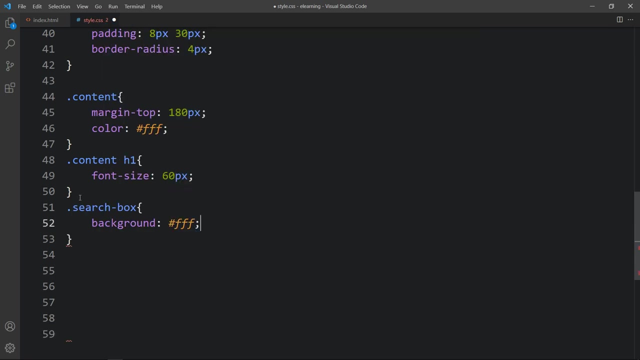 and here we will add h1 for this title. we will increase the font size, so i am adding 60 pixel font size. this text looks good. next we will design the search box. so copy this class name, write it here for this search box. we will add background: it is white. then we will add width, then display. 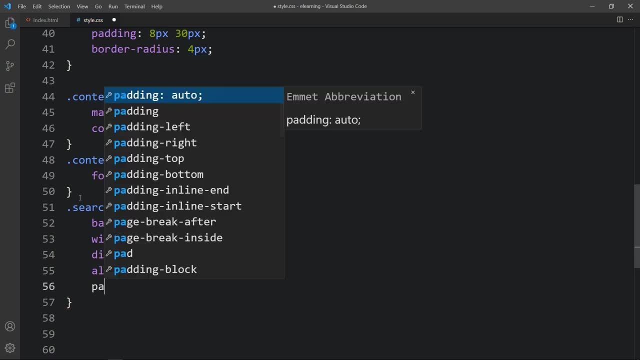 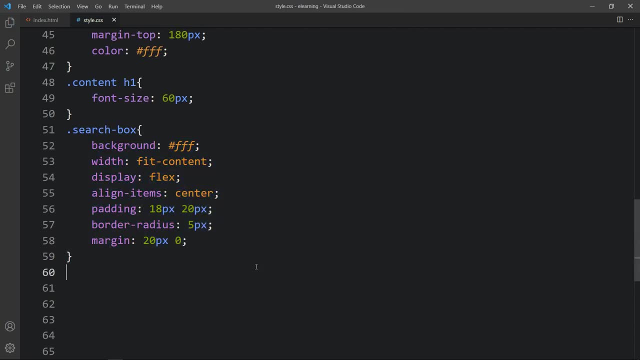 and align item center. then we will add some padding and border radius. let's add margin. now it looks like this: next we will design the input box and the icon. so let's come back and write this class name again and write input, because we have to design the input box here. we will add background, transparent, and we will 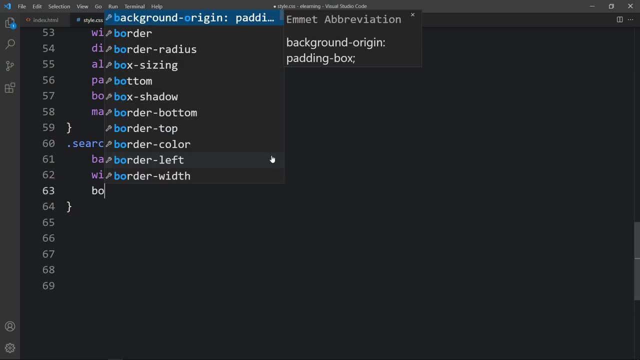 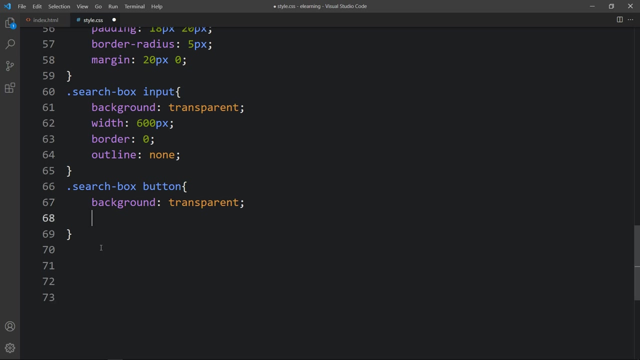 add width. let me add 600 pixel. then we will add border 0 and outline none. write this class name again and write button. for this button we will add background transparent. then we will add border 0 and cursor pointer. in this button we have added one icon using img tag, so here we will add. 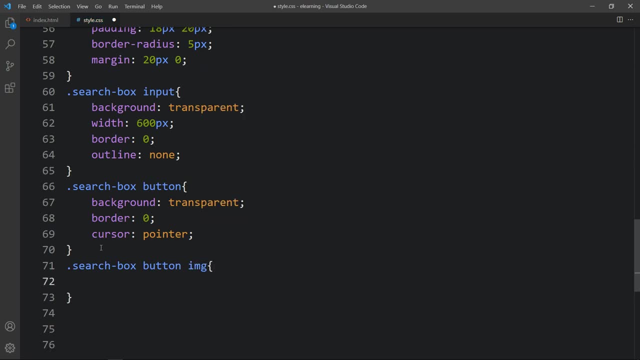 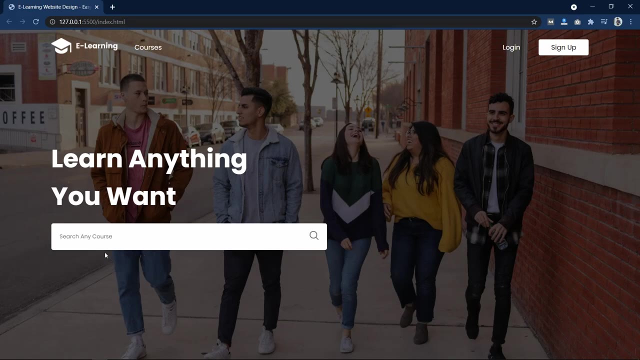 search box button img. for this image we will set the width. it is 22 pixel. now this search box looks good. we can write anything in this search box. after that we will add one text in tag. so let's come back and after this search box we will invite this picture. for this you can also. you are letting text beкими tag. come to select function menu at the top of deck, then click for addThis view dropbox. 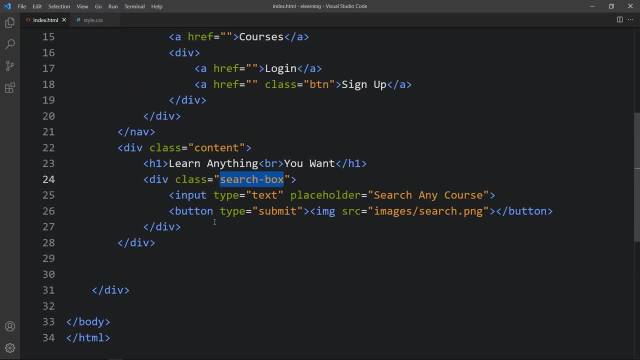 so let's come back and after this we will add search box button, cap name scanning using this search box option, in which you may see that compilations been downloaded automatically, so you can hit enter and enter function Asia. then, after this, let's come back and after this text text, IP tag, infotainment and popup Ihnenal tag that will be typed after: suppose ka. 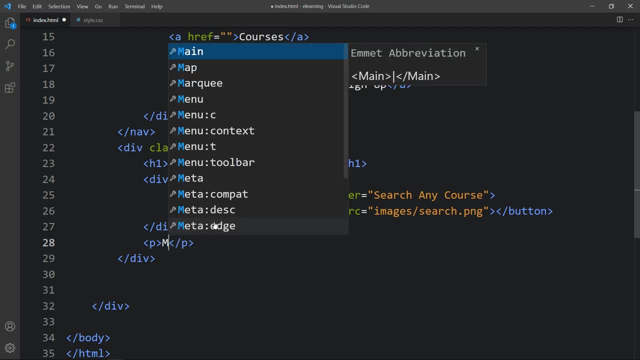 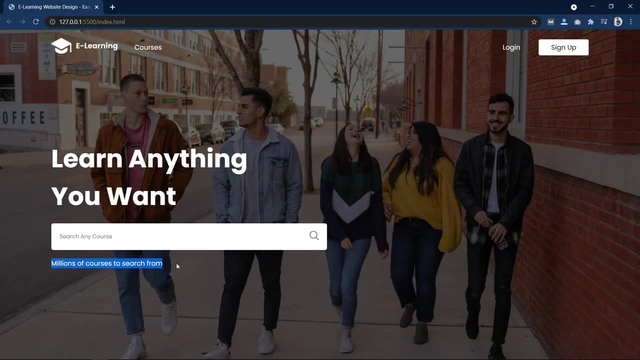 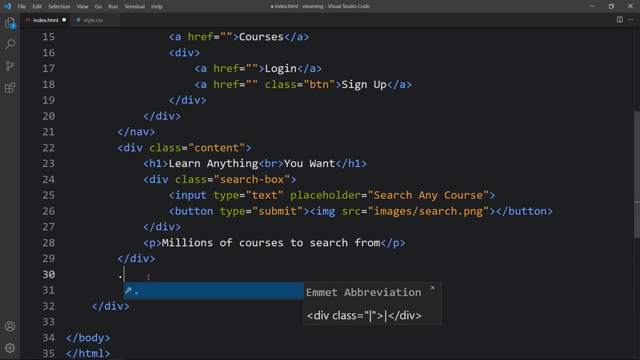 after this search box, we will add one p tag and we will add one text. it is millions of courses to search from. after this, we will add two icons, which is previous and next icon. so let's come back, and here we will create one div. let me add one class name arrow and 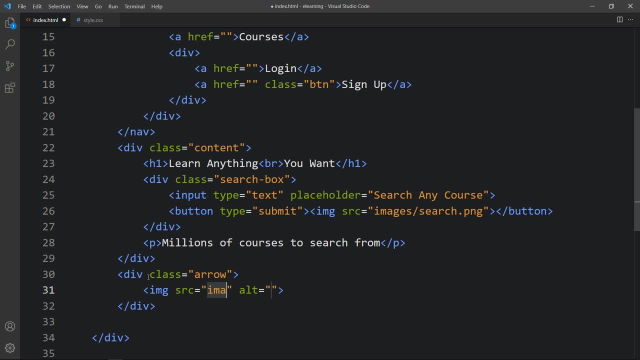 here we will add image. image file path. it is images slash- previous dot png. let me duplicate it and change the file name. it is next dot png. refresh the website and you can see these icons. next we have to add some css, so copy this class name arrow, write it here for this. 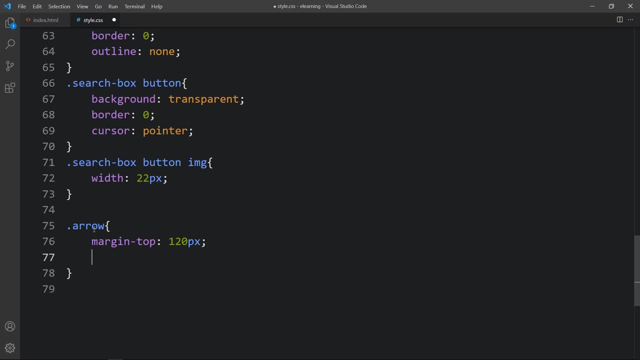 one. we will add some margin from the top, write this class name again, then write img and for this image we will add width: 15 pixel. then we will add some padding and we will add background rgba and this color code. then we will add border radius of 5 pixel. box sizing will be content box. then we will 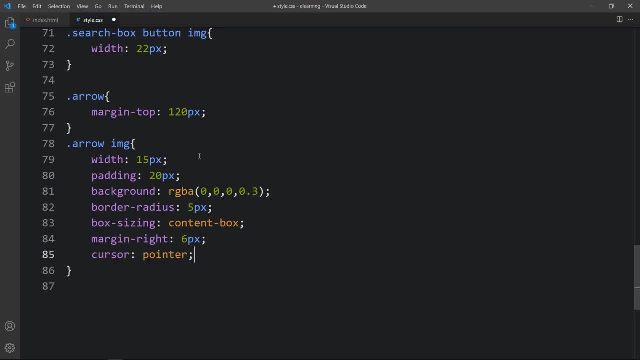 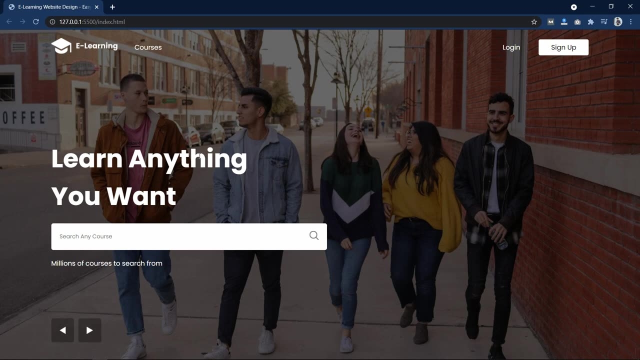 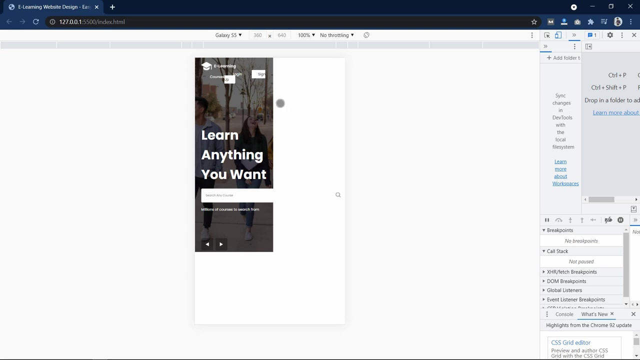 add some margin from the right side and cursor pointer. now this button looks good. now we have added all the contents on this webpage. next, let me change the screen size so that you can see this search box. width is very large, so let's come back and here. first we 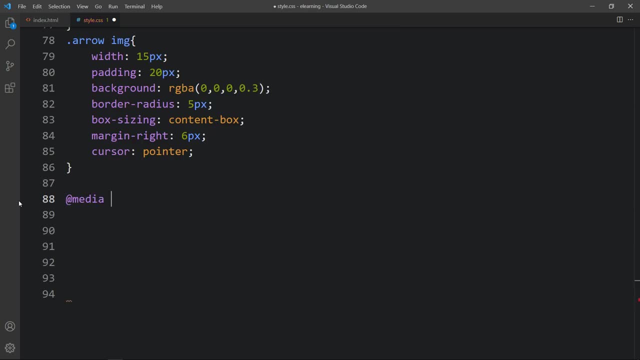 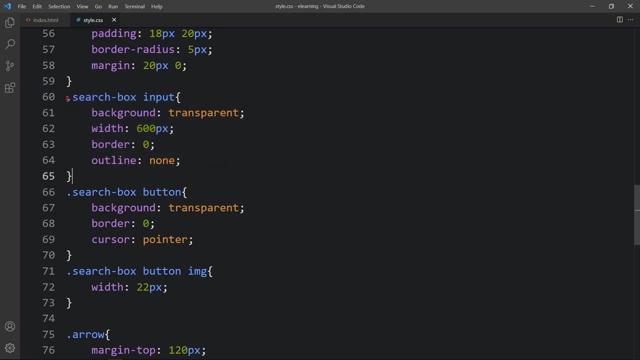 will add one media and here we will define the max width. let me add 700 pixel. so whatever css we will write in this media query, that will be only applicable for a small device whose maximum width is 700. so here you can see, in this search box input we have added width, 600 pixel, so we have to reduce this. 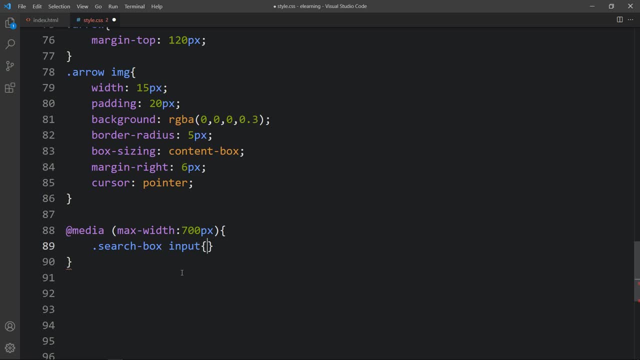 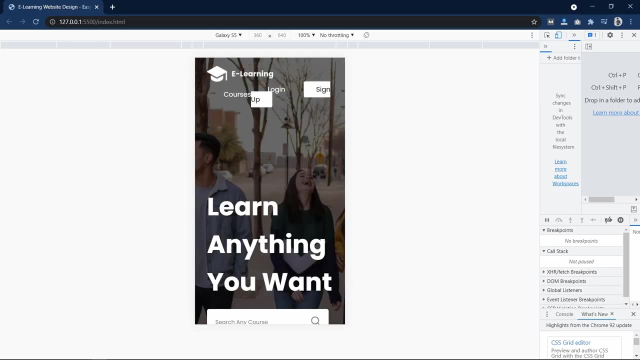 so just copy this one search box input, write it here in the media query and here we will set width, 230 pixel, which is a small width. now you can see the input box width is looking good. next we will design the top area, which is navigation bar, where we have added the logo. so let's come back and you can see we have added the. 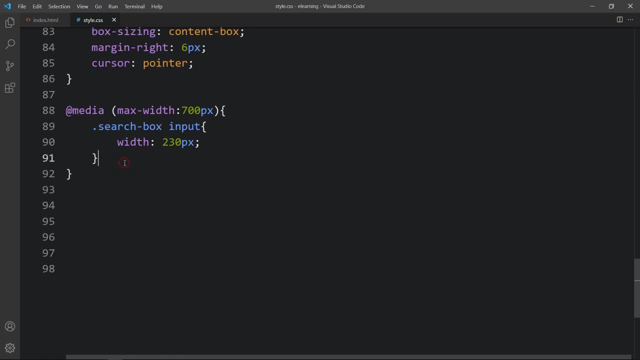 class name: nav logo. so write this class name in the media query. for this one we will add flex basis 100 percent, so it will use the complete space in the row and here we will add margin from the bottom 10 pixel. then we will add text align center so that the logo 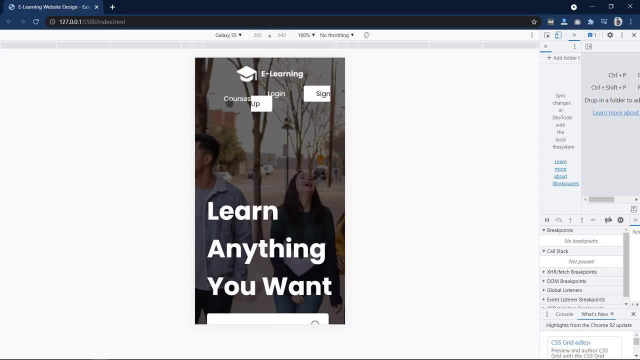 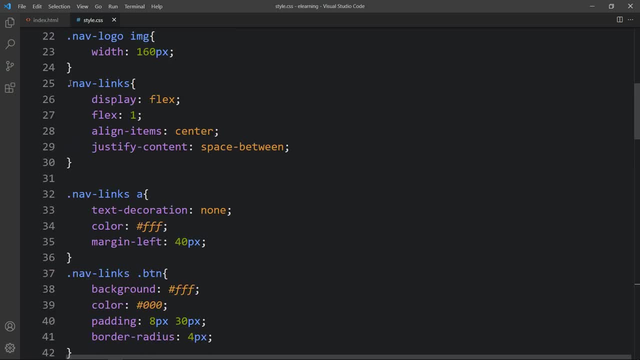 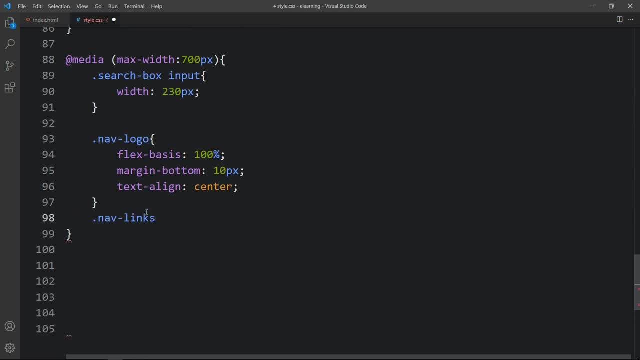 will be in the center. you can see this logo in the center. next we will design these links. let's come back and you can see we have added the class name nav links. so just copy this class name, write it here in this media query. here we will add justify content center and. 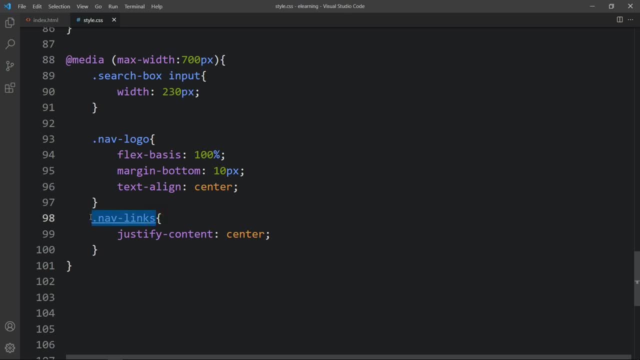 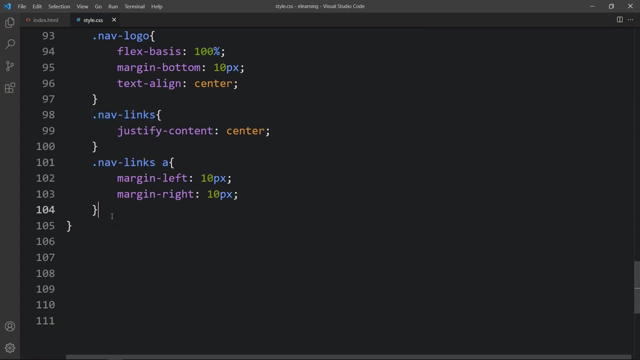 after that we will add this class name again and here we will add a tag for this anchor tag. let me add margin from the left side, 10 pixel, and same margin from the right side, 10 pixel. let's copy this class name again, then write dot: btn. we have added one btn class name for the last link for this. 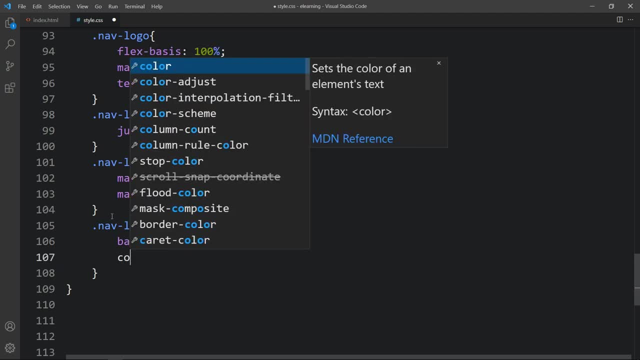 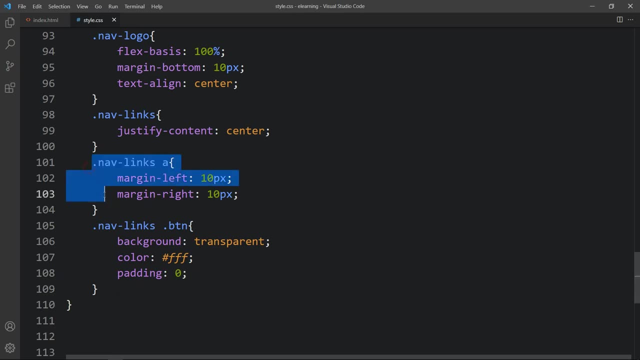 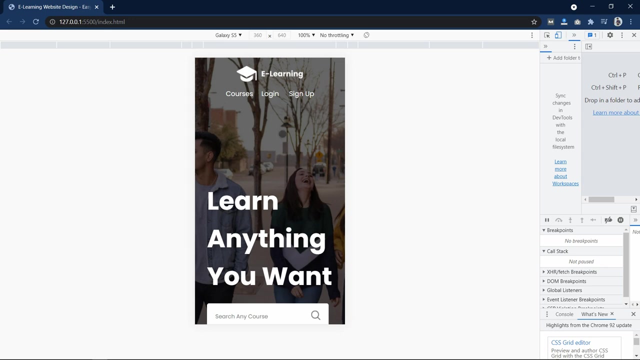 one. we will add background transparent and we will add the color. then we will add padding 0. after that, refresh the website again and you can see the top navigation bar looks good. there is a logo in the center. after that we have three links. next we have to reduce the size of this title. so let's come back and you can see. 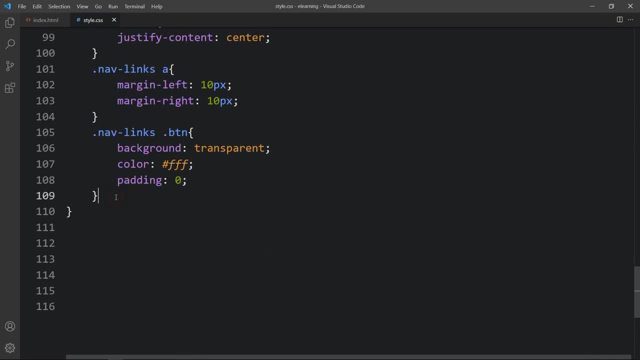 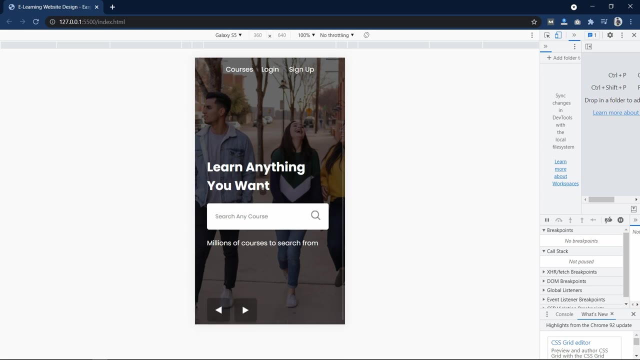 here we have added content h1. write it here in this media query and here we will decrease the size. it is 30 pixel now. you can see the font size looks good for the title. next we will reduce the height of this content. so let's come back, and here we will add the class name content and here 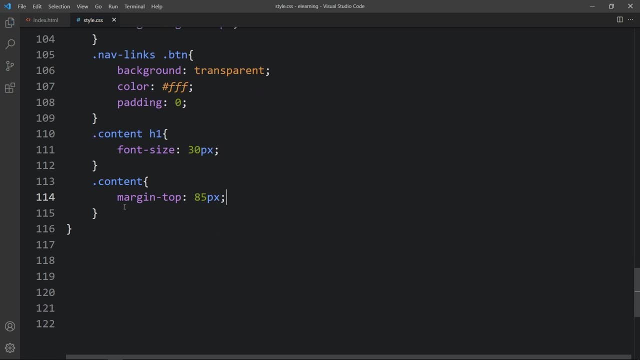 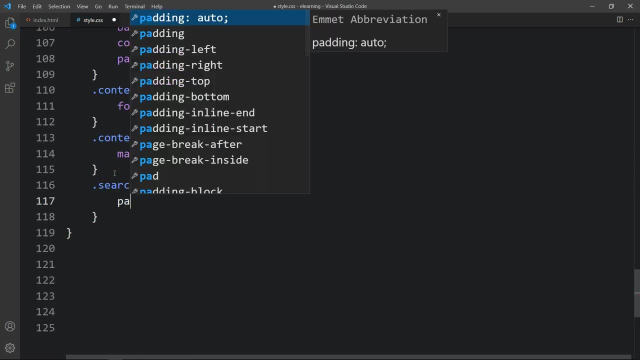 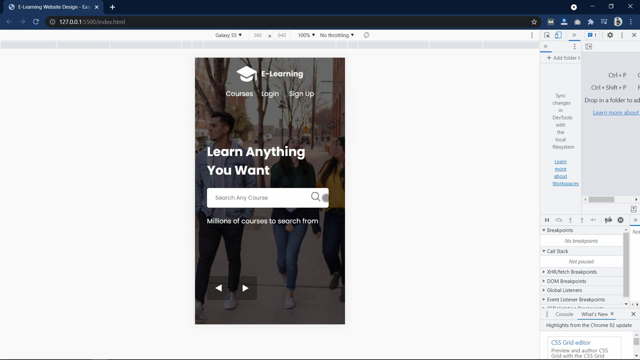 let's add margin from the top: 85 pixel. after that we have the search box. so you can see we have the class name here. write it here in this media query and for this search box we will add padding: 10 pixel, 20 pixel. now this search box looks good. 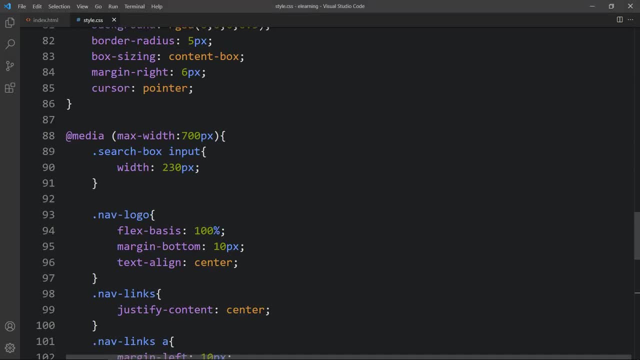 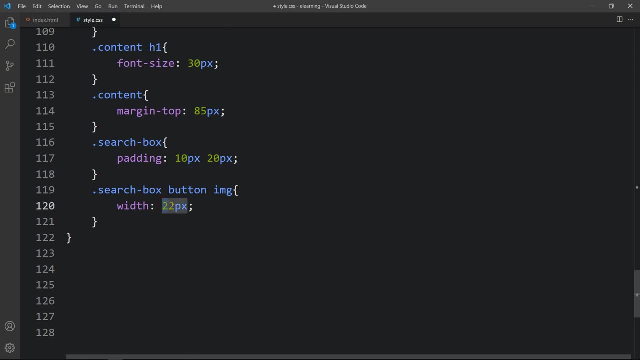 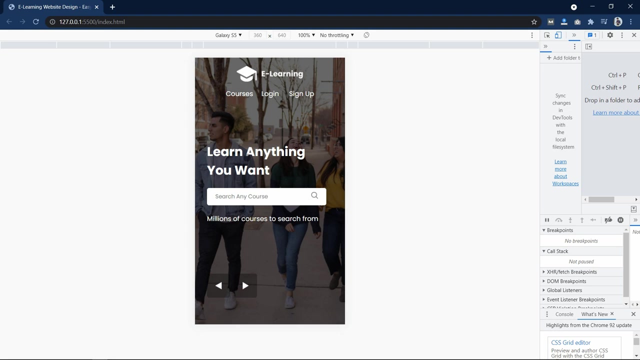 next we will reduce the size of this search icon. so just come back and you can see we have added this size here. just copy this one, write it here in this media query and here we will reduce the size 16 pixel. now this search icon looks good, so we have made this website. 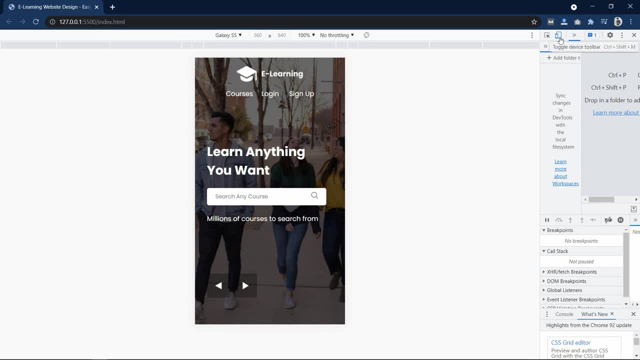 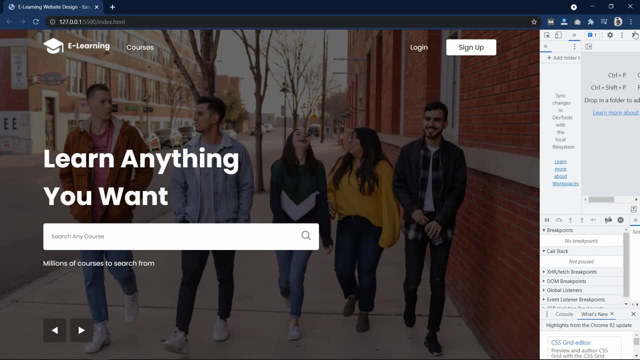 responsive for a smaller screen. let me change the screen size so that you can see it works fine. we have completed this web design using html and css. i hope this video will be helpful for you. if you have any question, you can ask me in the comment section. please like, and. 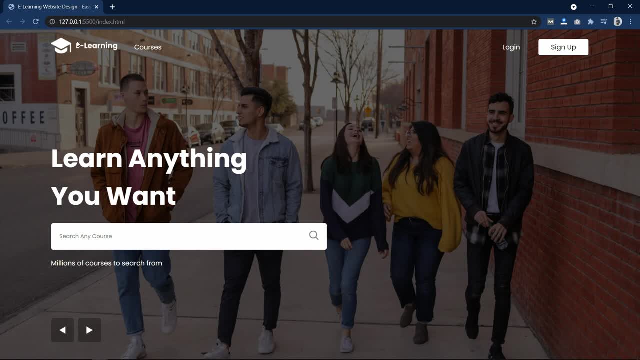 share this video and also subscribe my channel, ez tutorials, to watch more videos like this one. thank you so much for watching this video.